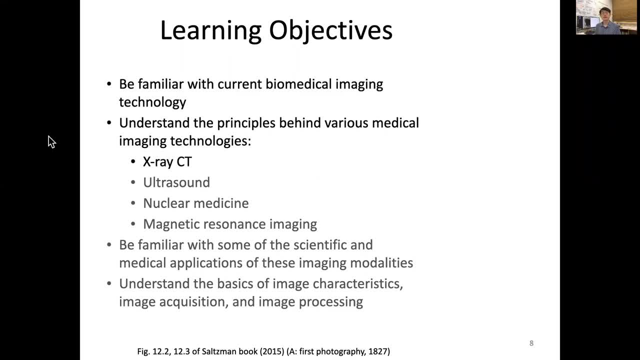 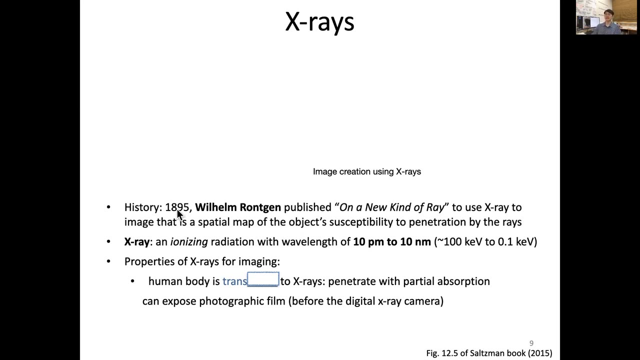 Hi, As a first medical imaging technique I want to discuss now x-ray and x-ray CT. So what is x-ray? There is a history that in 1895, Wilhelm Röntgen published a paper on a new kind of ray. that he doesn't know what that exactly means, And so he uses x-ray. 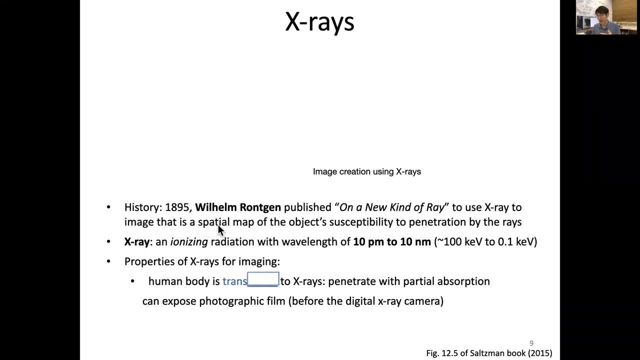 to image that as a spatial map of objects, susceptibility to penetration by that ray. So this is the schematic of conventional x-ray imaging. So what is x-ray, which is an ionized x-ray, and what is x-ray? It is the initial x-ray and it is the one that is coming back. 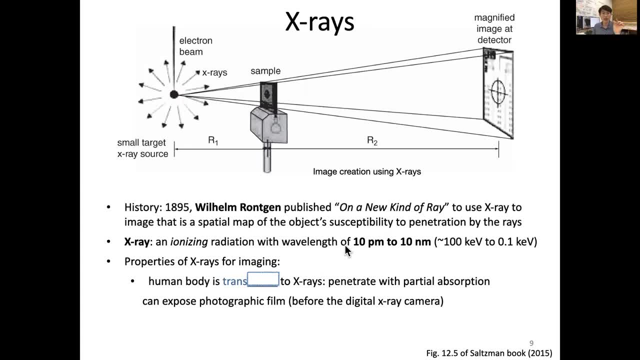 to us. The initial x-ray is a nice little image. And the initial x-ray is the initial x-ray is the image of an ionizing radiation, which means it's wavelength is quite short and the energy of this photon is pretty high, so powerful. So the wavelength is only about 10 picometer to 10 nanometer, Remember one: Ångström is the size of a hydrogen atom, So this is pretty pretty a short wavelength, meaning that the energy is high, so which the energy is almost 100 kilovolt per second. So this is pretty pretty a short wavelength. 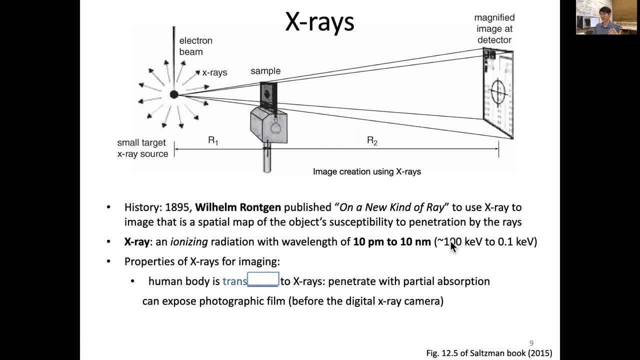 that means it is essentially the energy is high, so which the energy is almost about 70 kilos. So if you put a nuclear atom and it's the energy of a nuclear atom, electron volt, to about 0.1 kilo electron volt, so this it can hit the target and 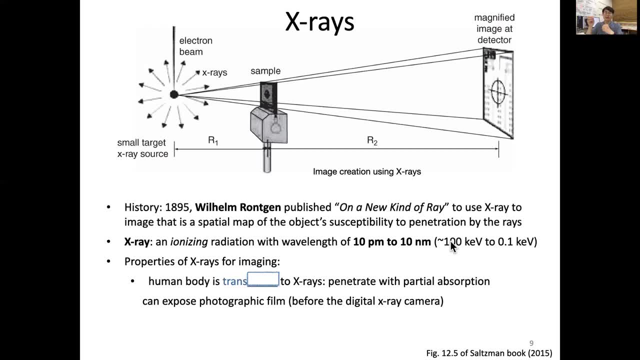 actually ionize, which means the it can eject electron, the valence electron, out of the, an atom. so, however, this is a can be useful medically. so you see, electron beam shoots a target which will send out x-rays outside, and this is so powerful that through the sample it penetrates. through the sample you can see it. 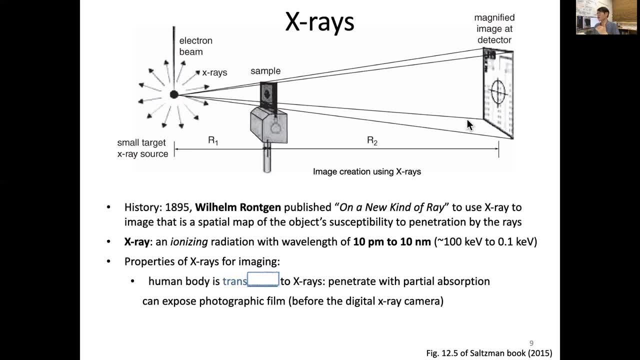 doesn't even bend or diffract, and so if you have a film on somewhere in distance, r2, then you can see a magnified images. so between this r1- r2, you can see r1 with respect to r1.2, plus r2 will be magnified. so the properties of x-ray for imaging is 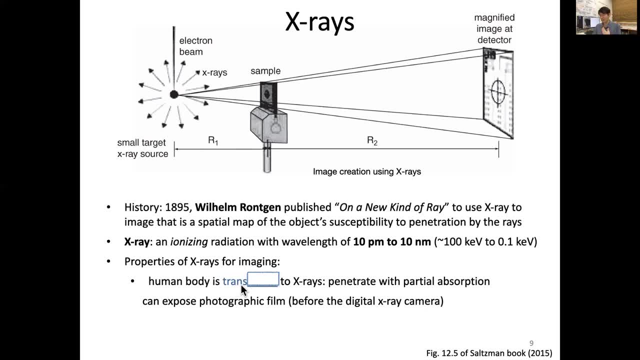 because our human body is translucent to x-ray, which means at the x-ray can penetrate with a partial absorption which can expose photographic film in the past and now we have digital x-ray camera. so translucent means it's in between transparent and transparent, an opaque. so that gives us a cool ways of looking first time through inside the 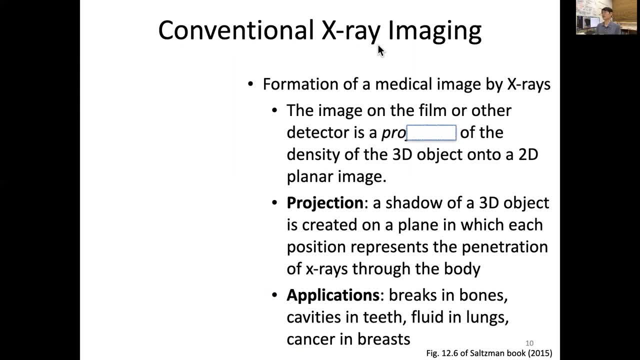 body. so conventional x-ray imaging is a formation of medical imaging by x-rays. so let me just explain conventional x-ray imaging as you see. there is an x-ray source or two, there is a x-ray coming up, there are filters and collimator making the x-ray direction into a parallel. in this particular case, then 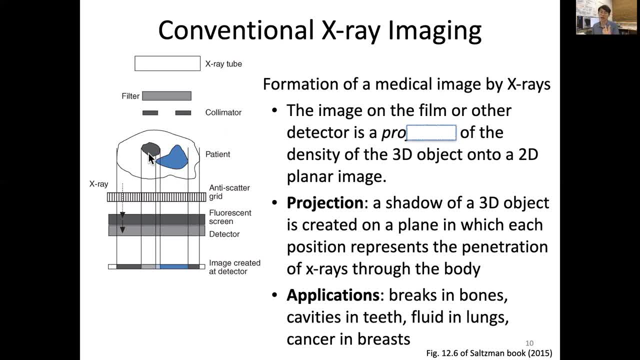 this is, let's say, a patient body, let's say this black one to represent a bone and this color represents some other organ. and that x-ray is penetrating because it's high, high energy photon. that it it actually we put as a ray, which means it won't bend. it just go straight and we have an anti scatter. 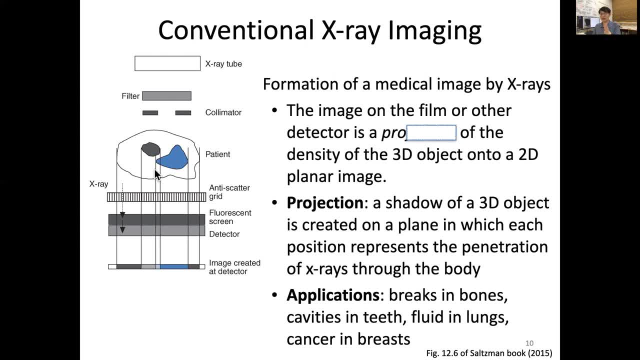 grid which blocks the scattered x-ray. so it passes through and it hits a fluorescent screen and that is a detector. so we can use either film or the it's a fluorescent screen- or we can image it using image creative at the detector so you can see that x-ray passing through. 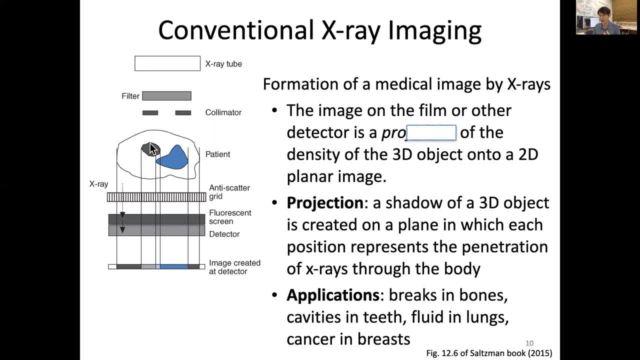 the x-ray direction. so we can see that x-ray passing through the x-ray direction. this part will be different contrast, because it has been observed much okay. so the image on the film or other detector is a a projection of the density map of the 3d object, but we are looking only to the planar or to the 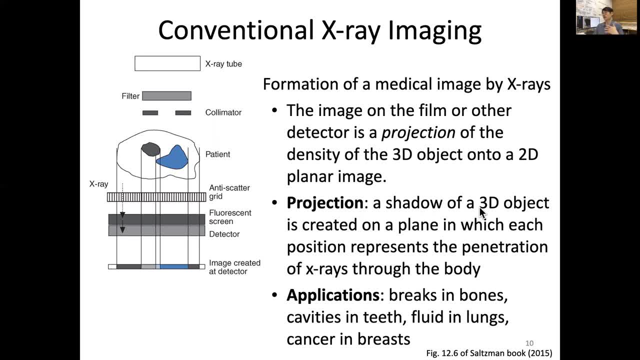 projection and the projection is a shadow of a 3d object. is created on a plane in which each position represents the shadow of a 3d object and the projection is a shadow of a 3d object. is created on a plane in which each position represents the. 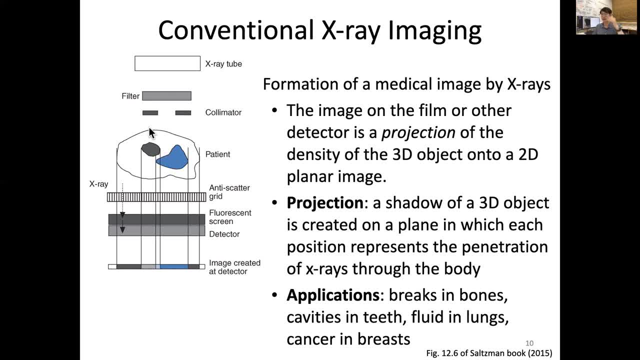 the penetration of x-ray through the body, the full penetration, and this simple two-dimensional projection has been very useful- that the applications include breaks in bones, cavities in teeth, fluid in lungs and even cancer in the breast. so i brought one example of my tip from dental x-ray. so you know, with this this is the x-ray source rotate through my face and it. 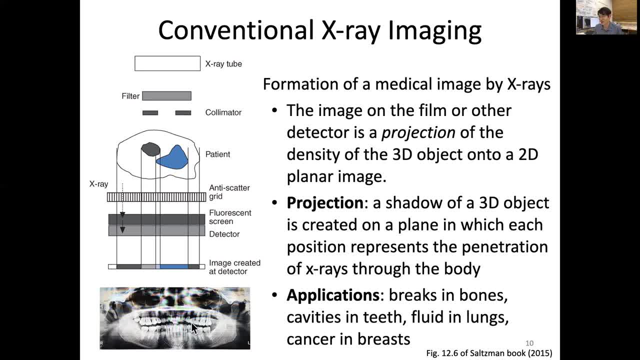 takes this x-ray figure and that particularly the dentist showed me that i have in this gap between this right, uh, side of my teeth and this happens to be the place whenever i ate some meal and there are, like foods and and depresses will be treated, kicking in inside. So after this, I understand the importance of flossing after meal, because 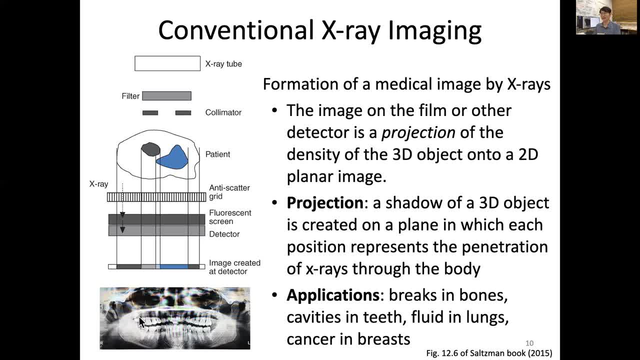 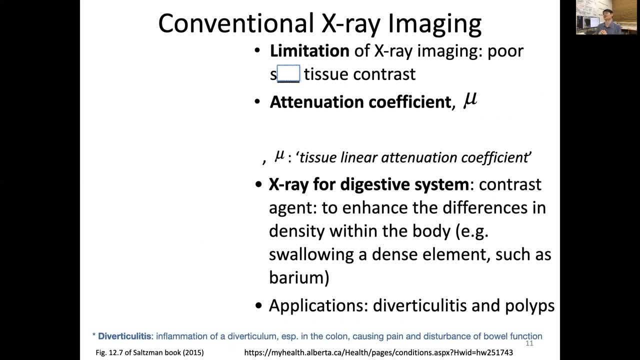 I realized this part is always. many times it has a problem. Okay, so conventional x-ray imaging has also limitations, and that's I want to show that conventional chest x-ray- here you can see a bones very well, but somehow you cannot see many things inside this lungs. 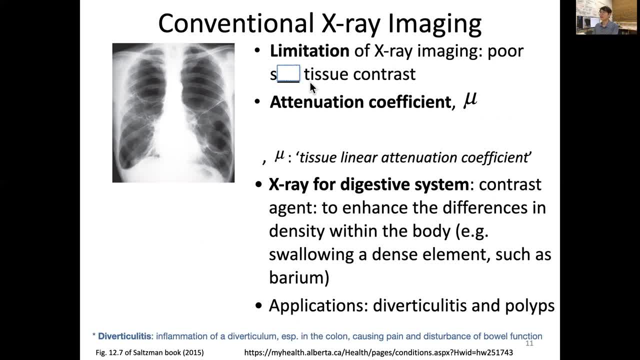 so very poor. so that is poor soft tissue contrast. So because the contrast mechanism is the absorption of the X-ray, where which is bone is the most easily absorbing the x-ray, So that we are based on this attenuation and we can have 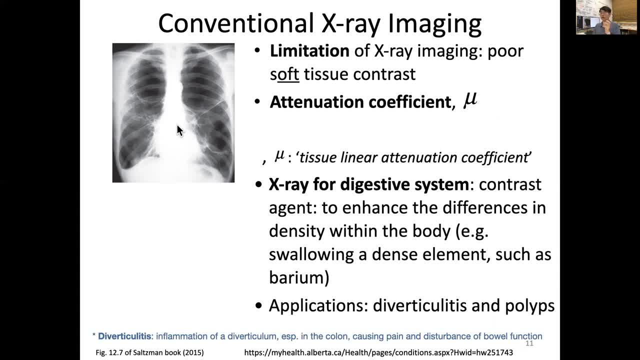 attention to the bone in the x-ray. So while this is so, it is not just bone, this x-ray coefficient for each of this tissue, So that original signal of N: zero. after, through this X amount of tissue that will be reduced by exponential decay. 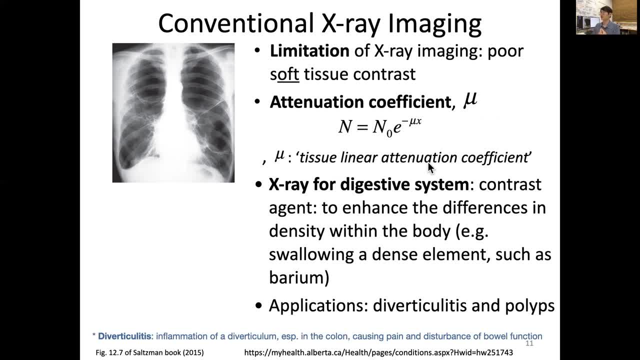 with N, So that mu is called tissue linear attenuation coefficient and you can see the unit will be one over length. So the example of x-ray for digestive system. and sometimes, because of this poor soft tissue contrast, we use a external contrast agent to enhance the differences in density within the body. 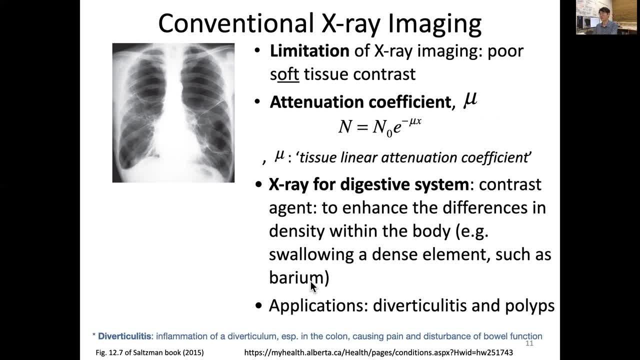 For example swallowing a dense element such as a barium, and then that can show the internal gut. So, for example, diverticulitis, which is a lydus, means inflammation in the diverticulum and sometimes a polyp, which is cancer pre-tumor. 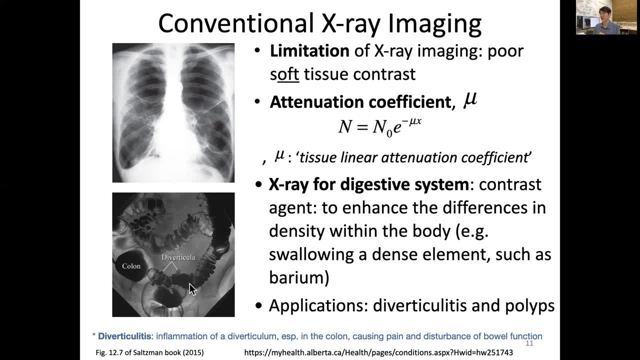 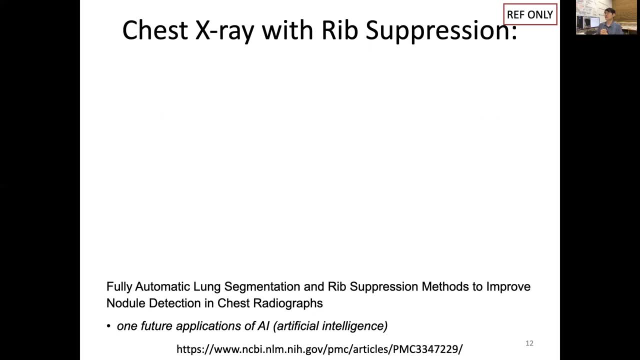 So the cancer inside colon can be detected by using this help of contrast enhanced x-ray. So I just bring some like nowadays, what's cool about this x-ray? for example, chest x-ray with rib suppression? because of the presence of the rib, we may easily miss some important regions inside the lung. 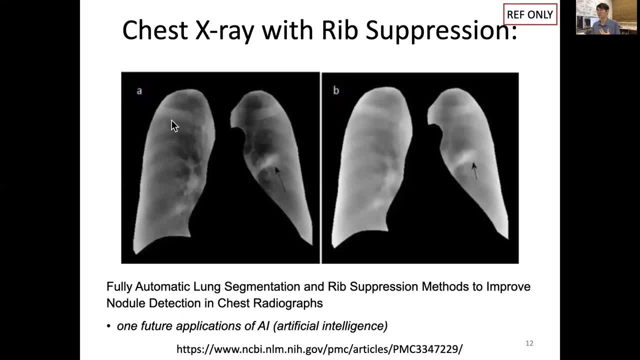 So this is just an example of a recent research that you see. this is the original. you can see the rib and one can do rib suppression and these regions may may work better. So fully automated lung segmentation and rib suppression methods to improve the nodular detection in chest X radiographs. 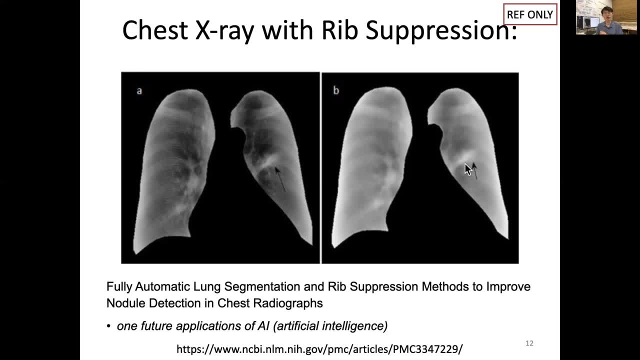 so that we can use machine learning nowadays, so that after that we can do lab prayers and other things. Here you can see the ready ran times. we can been highly impressed, and now we currently be in the naralan machine room, You can be that our body function is. 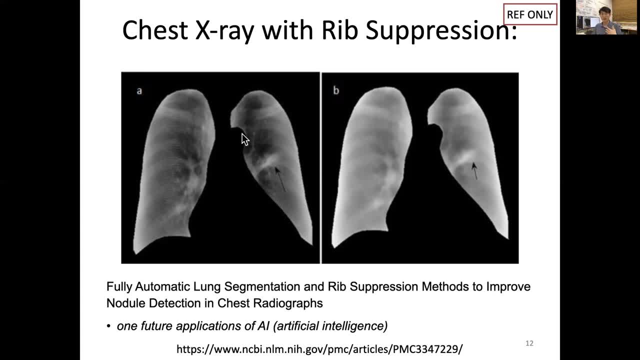 healing as well. there's a healing opportunity is steal into a tumor or see an X grade, since we got all this stuff from the muscles that are called limbs, but really salt, and a way to make sure that it not so bad. after sound enough of training, we can recognize this rib and then we 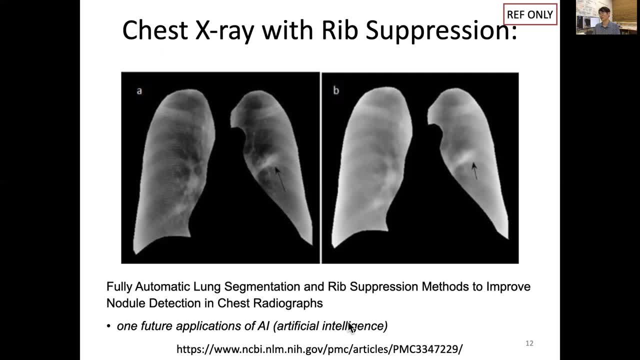 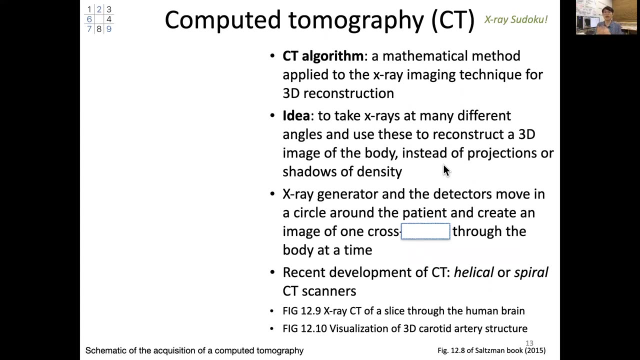 can remove that one by machine learning or artificial intelligence, which will allow a radiologist to detect small little changes easily. So now let's move on to a more advanced topic in X-ray, which is called computed tomography. You can consider it as a Sudoku of X-ray version, So you know. 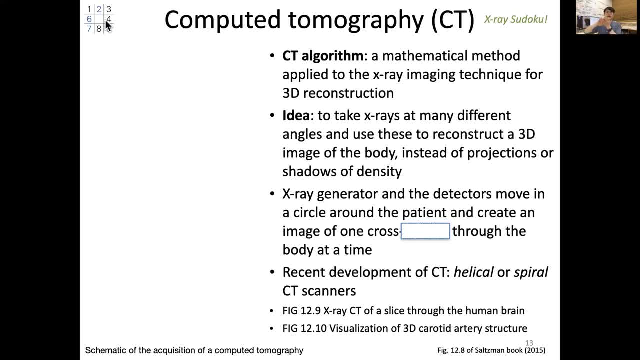 what Sudoku is, which is by having the resulting rule, you can fill out the inside, which, in imaging case, the inside a structure. So the CT algorithm is like a Sudoku: a mathematical method applied to the X-ray imaging technique. for the previous ones, 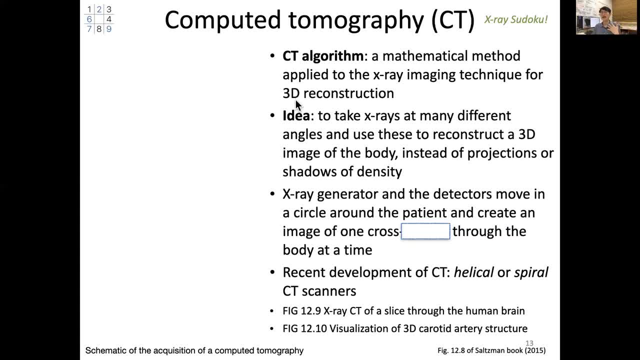 or 2D projection. Now we want to have a real 3D reconstruction. Reconstruction means because we only have 2D projection data like this and we want to see what number or what absorption of X-ray element will be here, So that we call. 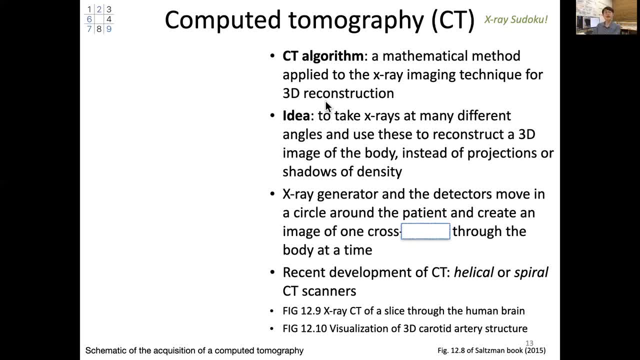 computed reconstruction. So idea is very simple. You just take X-rays as many different angles, Like Sudoku, you see different angles and directions to reconstruct the image of the body instead of projections of shadow, of density. So this is how. So X-ray source, like in this case, like fan, 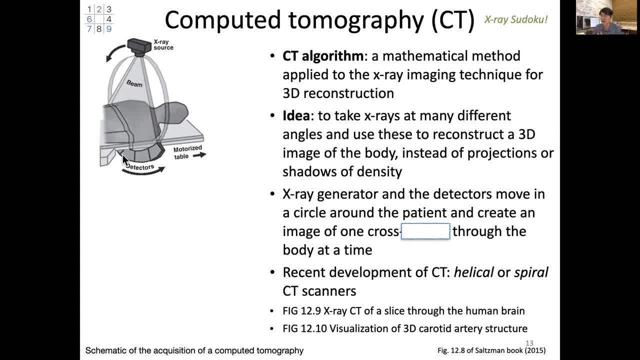 shape, X-ray beams passing through, so that you have a detector which is also arc shape, and then this will contain that projection information and you rotate them, So X-ray generator and detectors move in a circle around the patient and create an image of one cross, in fact section through. 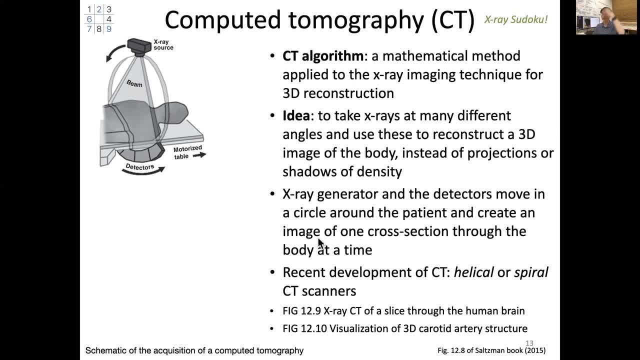 the body at a time. So one cross section, for example. we are looking at the brain section. Then here's an example. So you see, this is a brain section inside. it's not projection, it's a reconstruction And, as you see, there's a high contrast in the bone and a little. 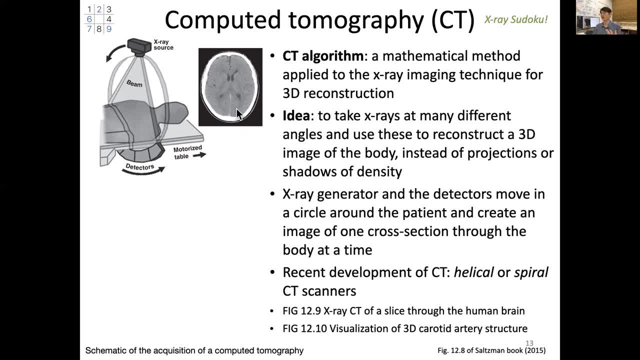 bit you can see vaguely for soft tissue contrast. however, after the CT, with a contrast enhancement, and now this is one, one slice, but you can make multiple slide to reconstruct the whole as a 3d, and that's a good example is here: this is a human, a bone in the neck, and here you see the contrast enhanced karate. 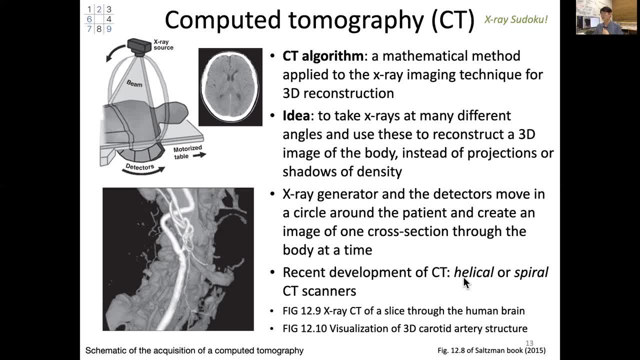 dolly. so this is possible by technology enhancement, by helical, like making these, this cross-section as a helical so that it can move faster or spider CT scanners. so this will allow us to find out the if there's any issues and problems inside our brain, our vessels, or our vessels in the carotid artery. 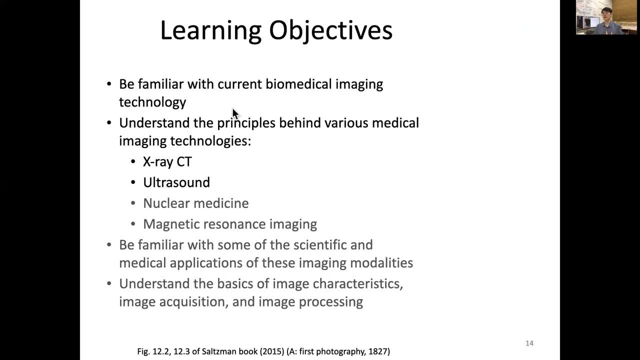 so next time I will discuss about ultrasound, and thank you very much for your attention.